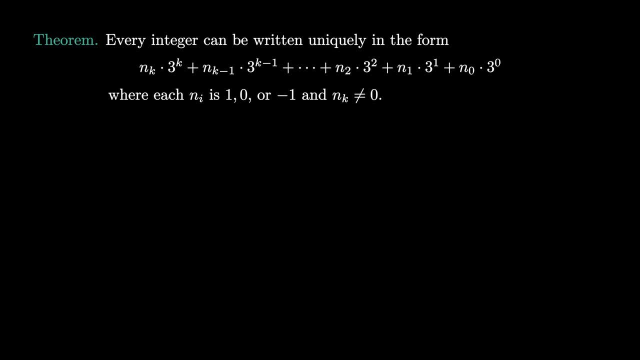 More formally that means n can be written as the form here, where n sub i is 1, 0 or negative 1 and the most significant digit, n sub k, is non-zero. This system is known as the balanced ternary representation, because the digits 1 and negative 1 are balanced around 0. It also works well because 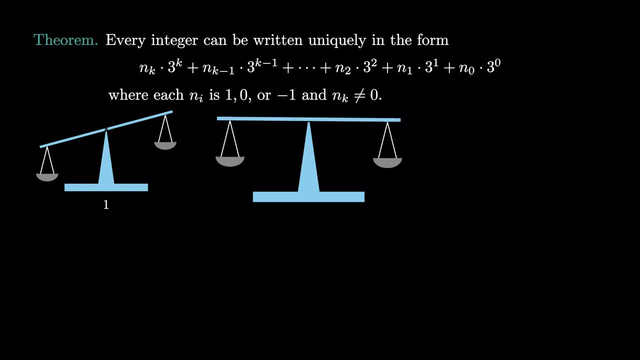 if our scale tips left, we'll call that a 1, if our scale tips right, we'll call that a negative 1, and if our scale stays balanced, we'll call that a 0.. So the three situations for a balanced scale are in with the digits for the balanced ternary representations. To see an example, we can check. 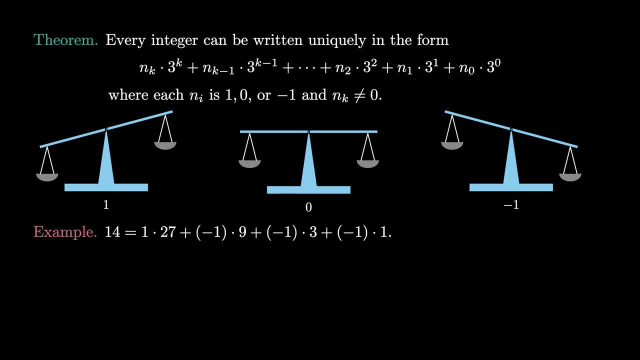 that 14 is 1 times 27, plus negative 1 times 9, plus negative 1 times 3, plus negative 1 times 1.. As we do with other positional numeral systems, we can simply leave off the powers of 3 and list. 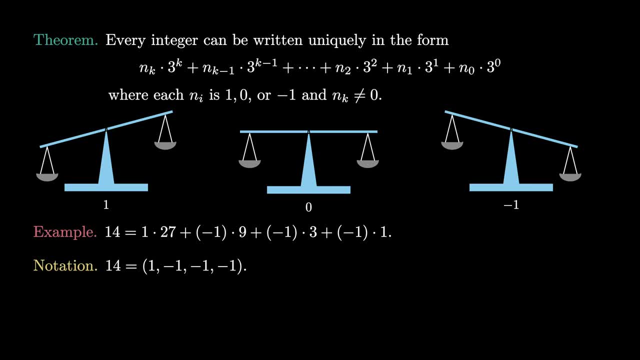 only the digits 1, 0 and negative, 1 in their appropriate positions. The position tells us what power of 3 the digits attach to. So 14 is 1 negative, 1 negative, 1 negative, 1.. A key feature to this numeral system is that we can also represent negative. 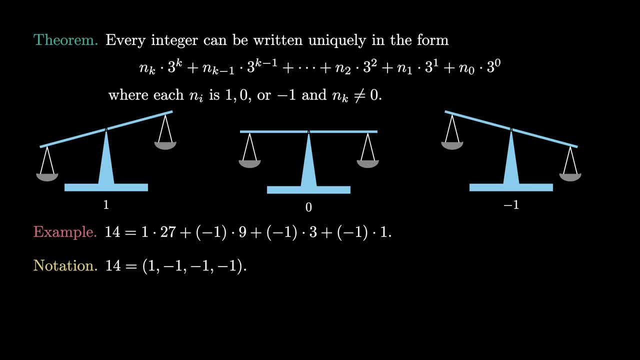 without adding extra information. To do this, we negate each of the digits in the corresponding positive representation. So, for example, negative 14 would be negative 1 1 1, 1.. Now that we know what balanced ternary representations are, let's see an algorithmic way to build such representations. 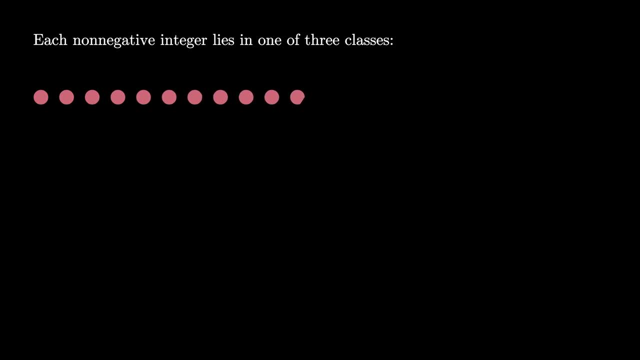 Each non-negative integer lies in exactly one of three classes. when considering divisibility by three, First you might have a number that's perfectly divisible by three and can be grouped in terms of threes. In this case we say there's a remainder zero when dividing by three. 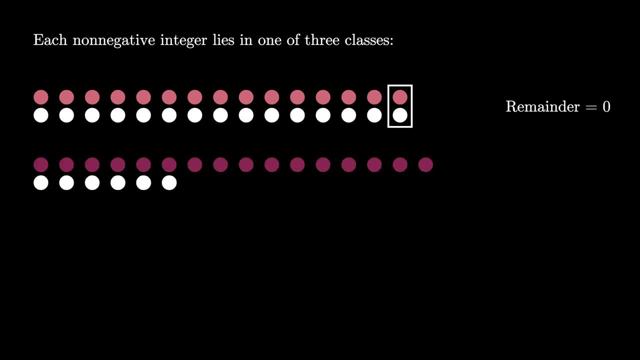 It may be the case that when you try to group by threes you have exactly one object left over. In that case we say: the remainder is one. Here's the strange one: If you have two pieces left over when dividing by three, you can actually consider that one extra copy of three. but now you have a 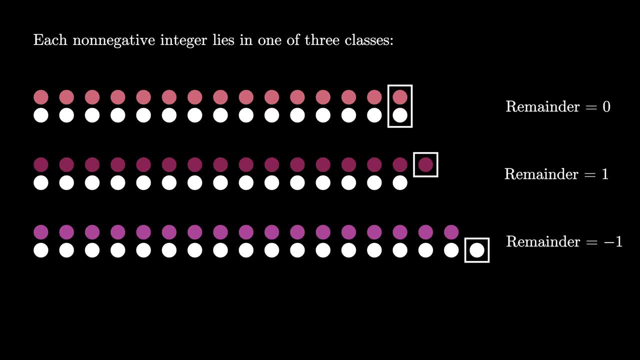 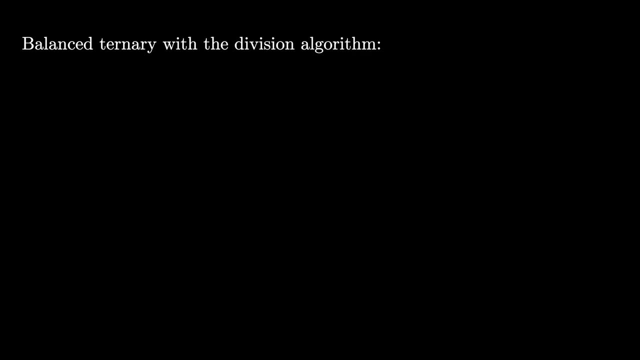 remainder of negative one. This observation leads to a modified division theorem stating that any non-negative integer, n can be written uniquely as n equals three, q plus r, where r is minus one, zero or one and q is an integer. Here's the general idea for repeatedly using the modified division. 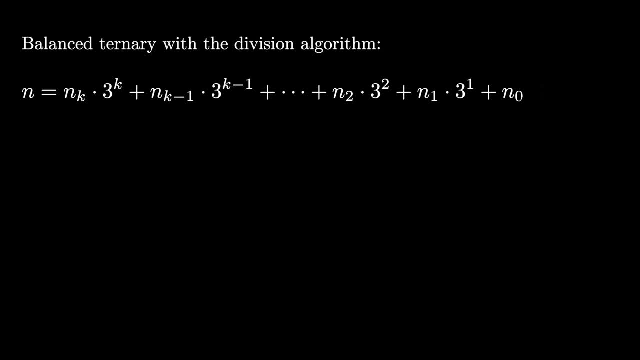 theorem to find the digits of the balanced ternary representation. Suppose we have n in its balanced ternary representation. When we factor out a three, we're left with the quotient and the remainder, which is n, zero or the least significant digit. Now we can repeat the process on the first quotient, q1.. 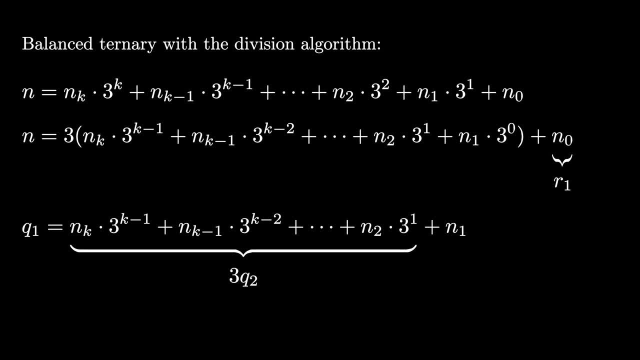 We see in this case, if we factor out a three, we have three times the second quotient and the remainder, which is now the digit attached to three to the one in the original number. We can repeat this process until we get a quotient. qm equals zero. At that point, the list of the remainders. 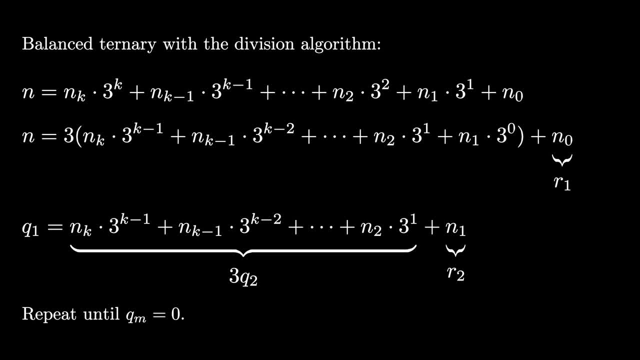 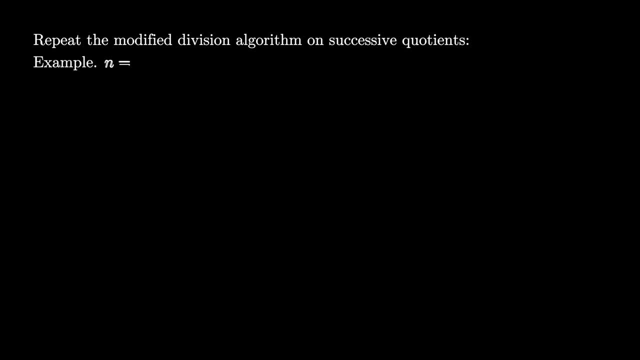 along the way will be the list of the balanced ternary digits from least significant to most significant. Let's see a visual representation of this repeated process using the example of n equals 20.. First we see that when we have 20 dots we can group together seven copies of three to overshoot. 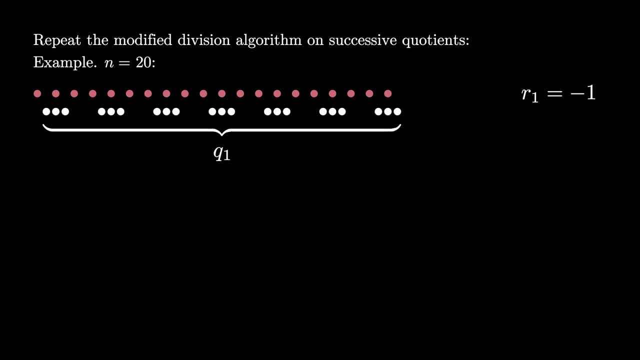 by one, leaving a remainder of negative one. Now we group those seven copies together so that our first quotient is seven. We use two copies of three, leaving a remainder of one on those seven. Group our two copies of three together for our next quotient overshoot with one three to give a remainder of negative one, leaving us with a. 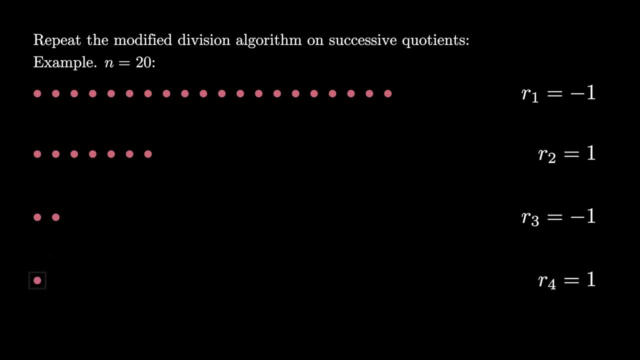 quotient of one, giving a remainder of one, so that our final quotient is zero, telling us we're done. This means that our balanced ternary representation for 20 is one, negative one. one and negative one. We read from bottom to top, because the division process produces the digits from least significant. 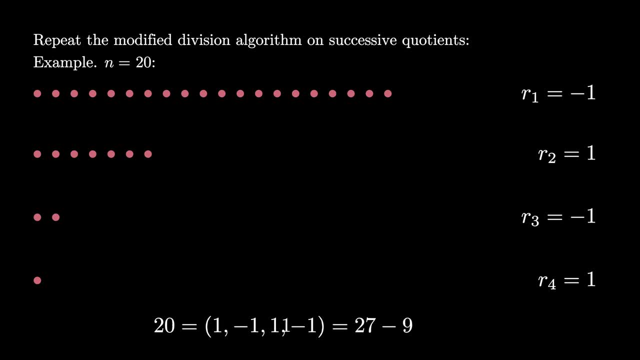 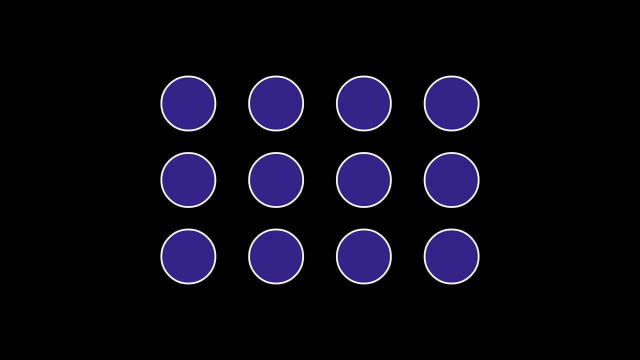 to most significant and we can check that 20 is 27 minus 9 plus 3 minus 1.. Now let's see how to solve the coin weighing problem. We can start with our 12 coins and we can give each coin a number from 1 to 12.. Then we're going to go through and we're going to 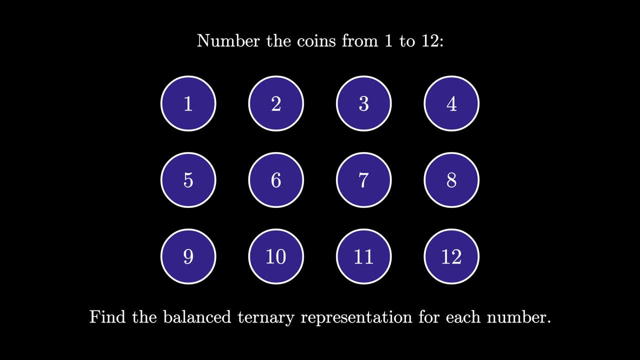 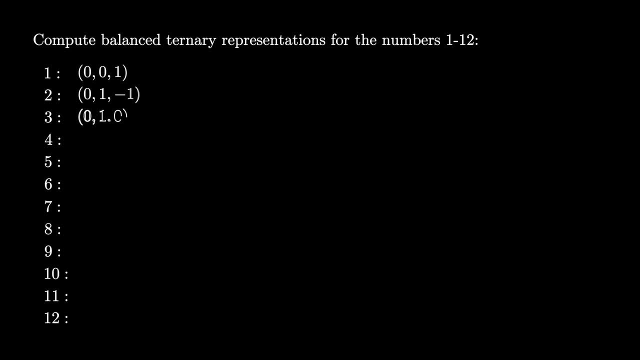 find the balanced ternary representations of each number from 1 to 12.. It doesn't take too long to compute these 12 balanced ternary representations by hand, but here they are for your reference. You can see, for example, that 10 equals 9 plus 1.. Notice also that 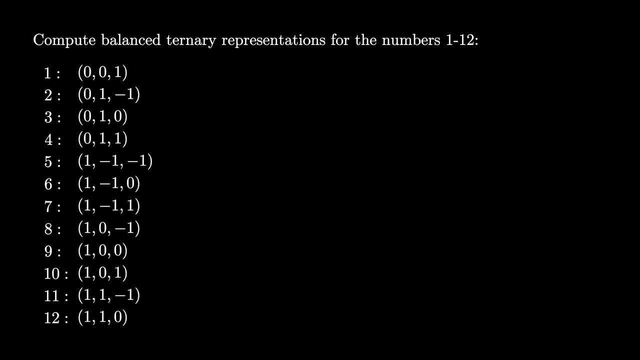 we've padded zeros at the beginning of the first four numbers shown here, so that each number has a balanced ternary representation with exactly three digits. Now, when we look position by position, something interesting happens. In the ones position or the ones digit, there are four. 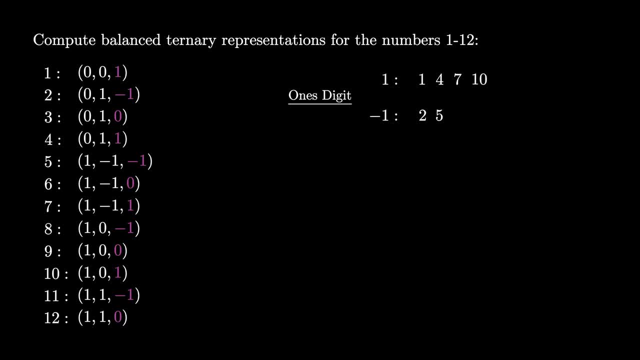 numbers that use a digit of 1,, there are four numbers that use a digit of negative 1,, which means there are four numbers that use a digit of zero. In the threes digit, however, it's a little bit different. In this case, there are five numbers that use a digit of 1, and there are only three. 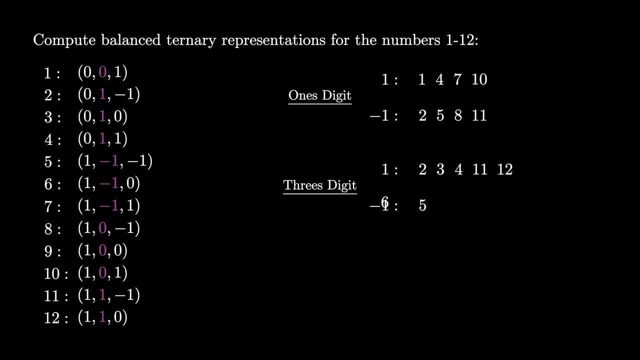 with a digit of negative 1,, but there are still four numbers using a digit zero. And in the nines digit or the nines position, it's even a little worse: There are actually eight numbers using a digit of 1, and there are zero numbers using a digit of negative 1,, but there are still four. 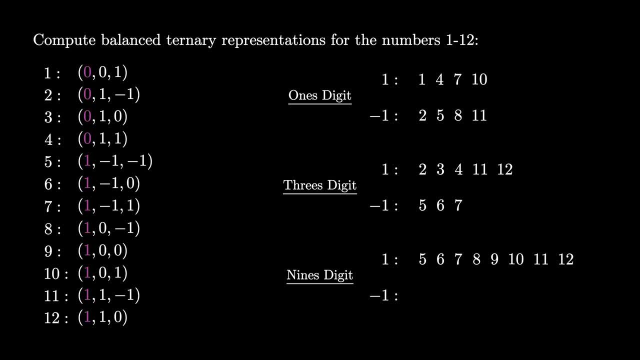 numbers using a digit of zero. It turns out we can make a slight modification using the fact that we can represent negative numbers in balanced ternary. We strategically negate the numbers 7,, 9,, 11, and 12 by negating all of their digits. Now, when we do this and we check position by position, we see: 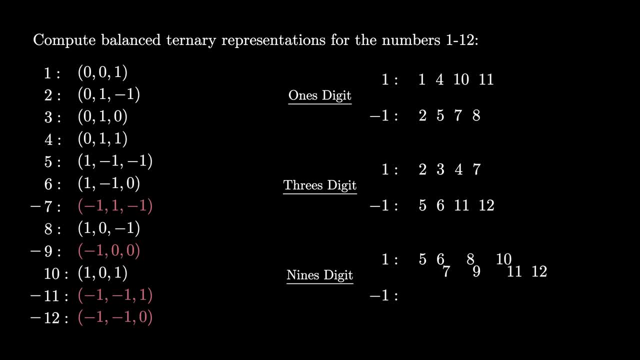 that in each position, there are exactly four numbers with a digit 1,, four numbers with a digit 0, and four numbers with a digit negative 1. A perfect balance that we can use to our advantage. In fact, we'll construct our weighings, one for each position. We'll put a coin on the left if 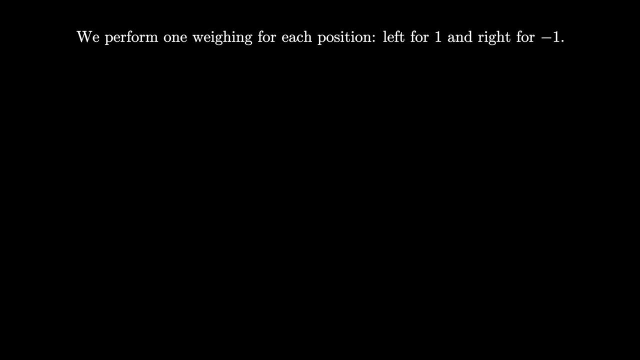 it has a 1 in the position and on the right, if it has a negative 1 in the position, We'll leave the coin off if it has a zero. So, using our balanced ternary representation, here are the three weighings we get One for the ones digit, one for the threes. 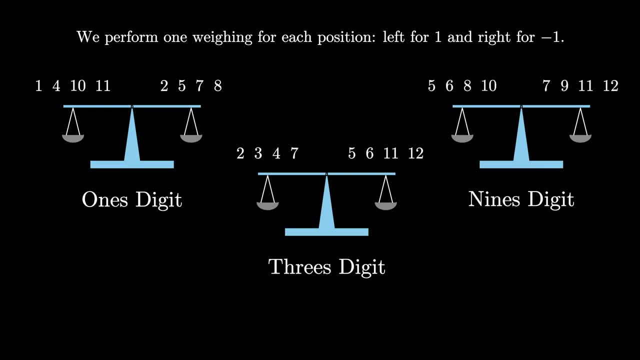 digit and one for the nines digit. We can then read off the three weighings as the balanced ternary representation of an integer, and that number will be the identity of the counterfeit coin. We will know that the coin is heavier than the rest if that number matches the number from. 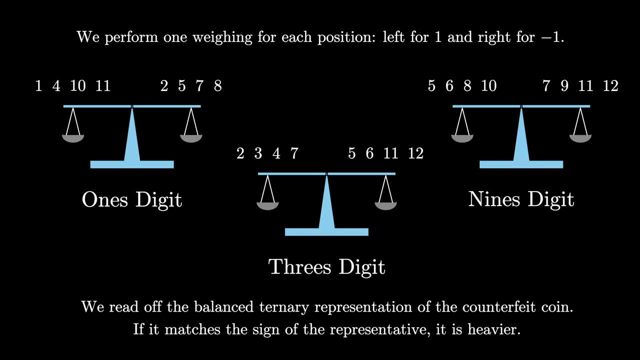 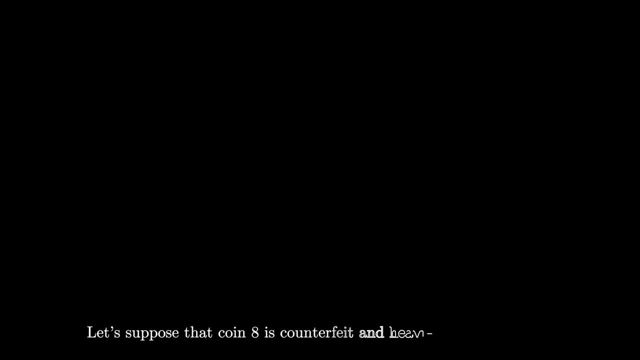 the list of representatives we used, or it will be lighter than the rest, if it's negative, of the representative that we chose for our balanced ternary representations. Let's see this process in action, where we suppose that coin 8 is counterfeit and heavier than the rest, Our 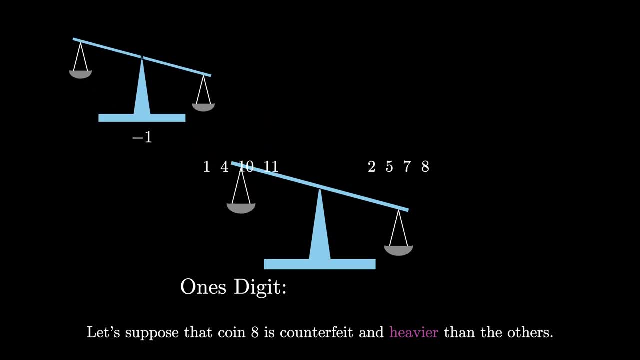 first, weighing for the one digit will point to the right, because that's where 8 is giving a digit of negative 1.. For the threes digit, we see 8 is not here in our weighing, so the balance balances and we get zero for our digit. And finally, for the nines digit, 8, is on the left. 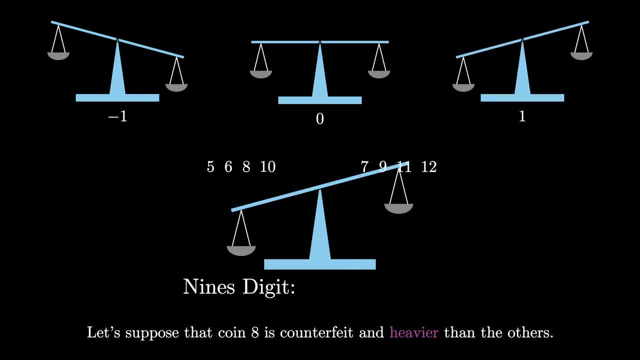 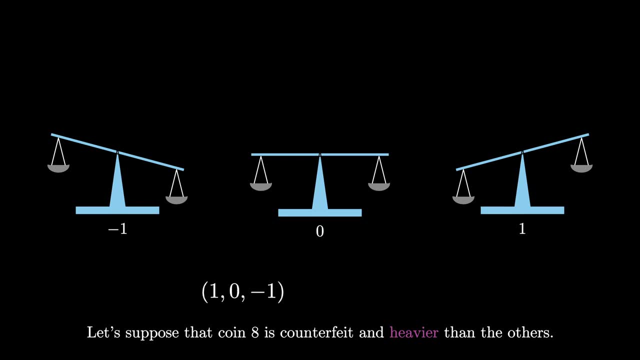 so the scale points left and produces a digit of 1.. From these three weighings we read right to left to see that our balanced ternary representation is 1, plus 0, negative 1,, which equals 9, plus 0, minus 1, or 8.. When we check our representative list, 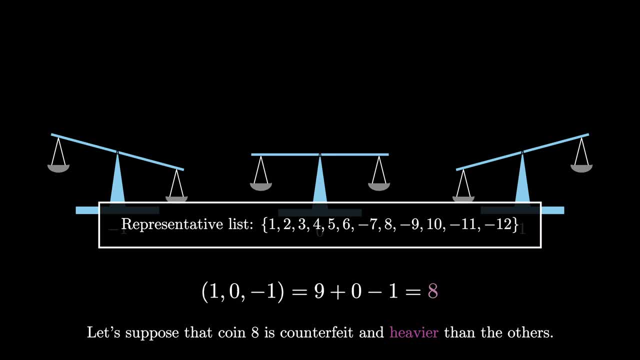 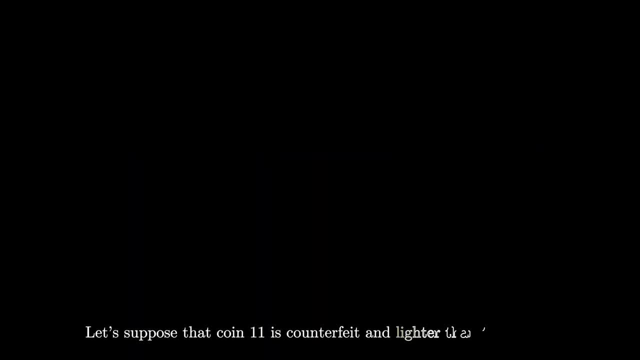 we see that 8 is positive and since that matches what we found, we know that coin 8 is counterfeit and heavier than the rest. Let's check another example where coin 11 is counterfeit, but this time lighter than the others. For the ones digit weighing, we see 11 on the left. so the scale tips. 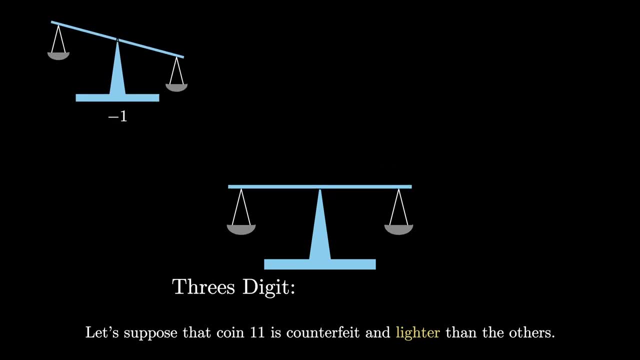 right, giving a digit of negative 1.. For the 3's digit, we see 11's on the right, so the scale tips left, giving a digit of 1.. And finally, for the 9's digit weighing, we see 11 is on the right, so the scale tips. 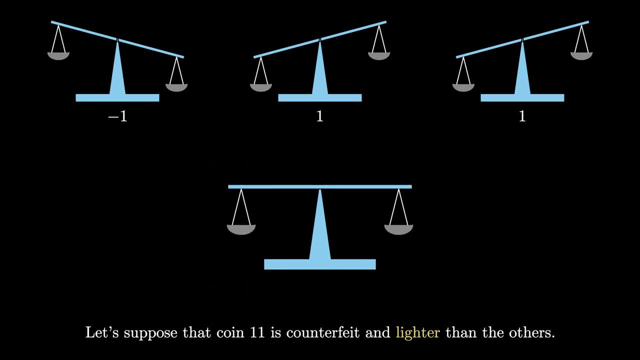 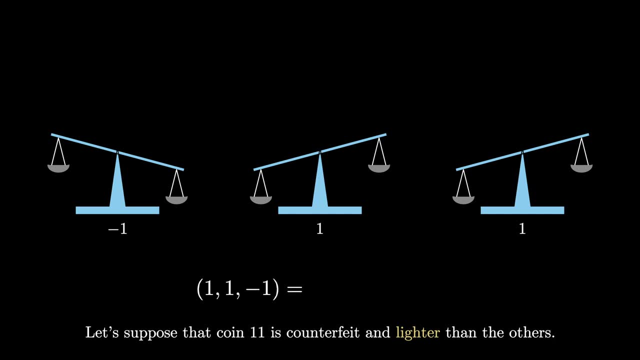 left, again giving a digit of 1.. Using these three weighings, we get our balanced ternary representation, reading from right to left, of 1, 1,, negative 1,, which corresponds to 9, plus 3,, minus 1, or positive 11.. 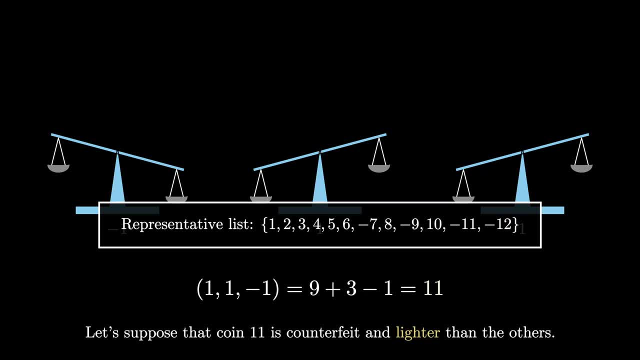 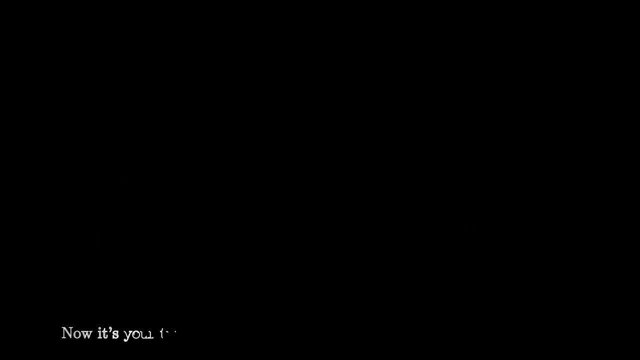 But remember, 11 was one of the numbers that we negated for our representative list, so we know that coin 11 is counterfeit and this time it's lighter than the others. Now it's your turn. Can you determine which coin is counterfeit and if it's lighter or heavier than the? 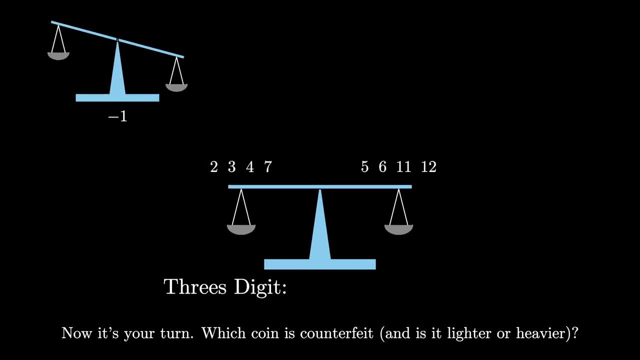 rest, if we get the following three weighings: The first two weighings both tip to the right and the final weighing stays perfectly balanced. Just remember that our weighings move from least significant to most significant. Just remember that our weighings move from least significant to most significant. 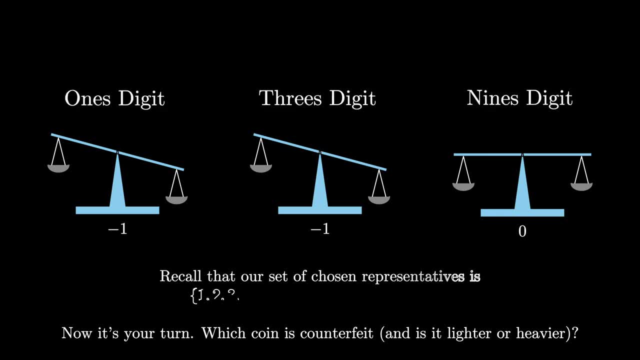 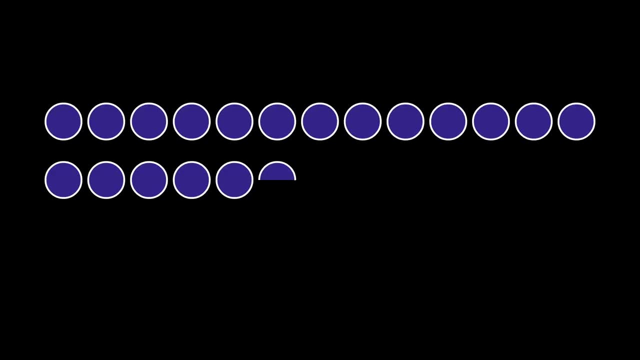 Just remember that our weighings move from least significant to most significant as you go from left to right, and recall that our set of chosen representatives only negated the numbers 7,, 9,, 11, and 12.. With this solution in hand, the more challenging problem is actually not that much harder. 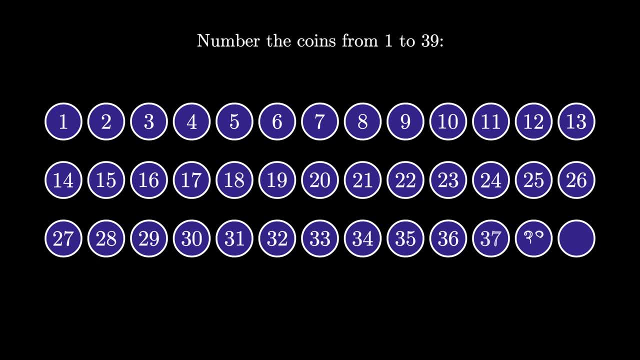 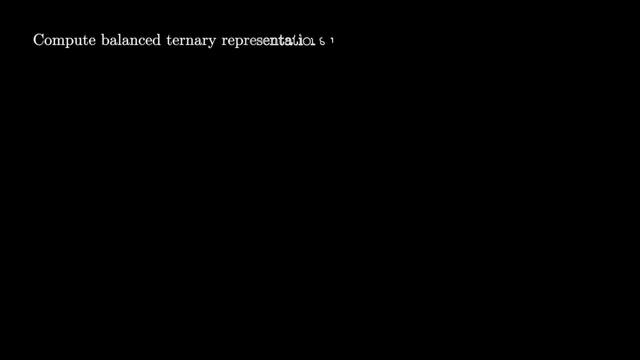 When we have 39 coins, we can number the coins from 1 to 39, and then again we can find the balanced ternary representations for each number. You can work out these representations by hand and it doesn't take that long. but 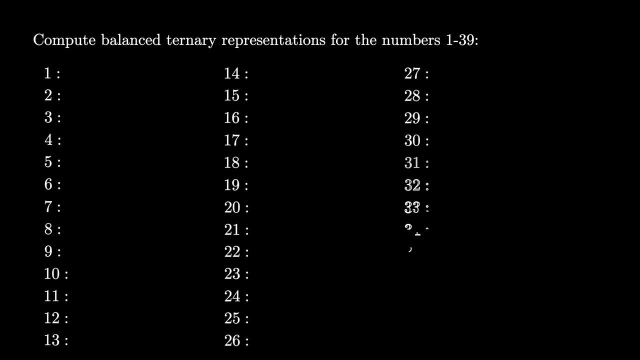 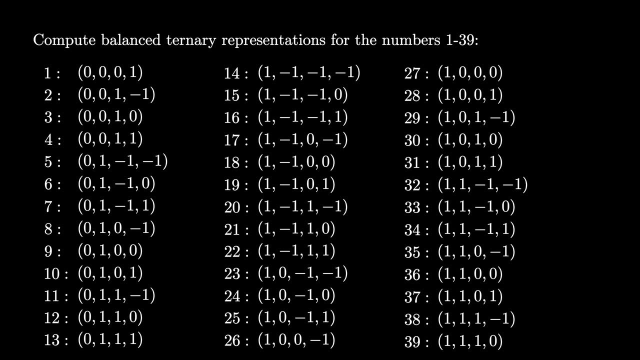 here's the list again for your reference. In this case we pad 1,, 2, and 3.. We pad representations with zeros at the beginning so that each representation between 1 and 39 has 4 digits. Once again, there are 13 numbers using a digit of 1 in the ones position. 13 numbers using 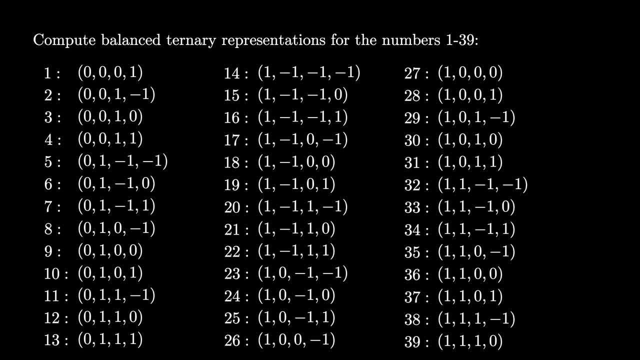 a digit of negative, 1 in the ones position and 13 numbers using a zero in the ones position. Unfortunately, this doesn't happen in the three other positions as well: the 3s position, the 9s position and the 27s position. 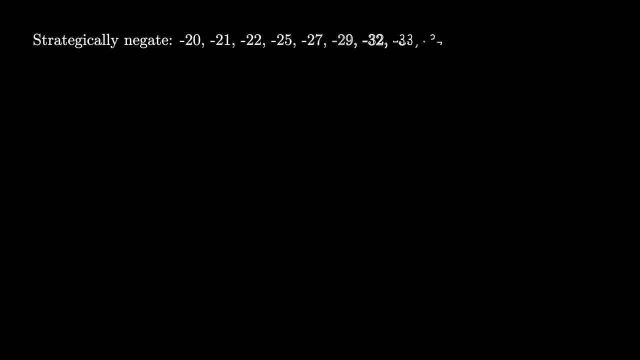 But, similarly to what we did last time, we can strategically negate 13 values. When we do these 13 values as shown here, we can strategically negate 13 values. When we do these 13 values as shown here, we can strategically negate 13 values. 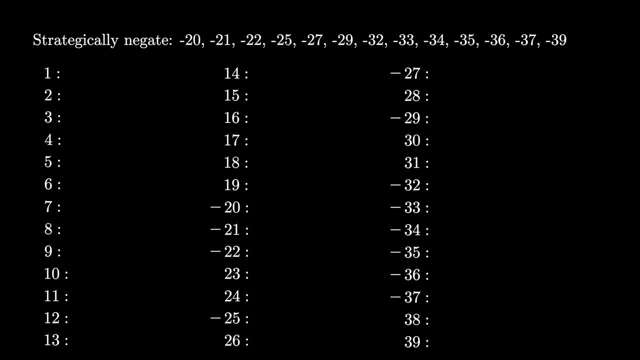 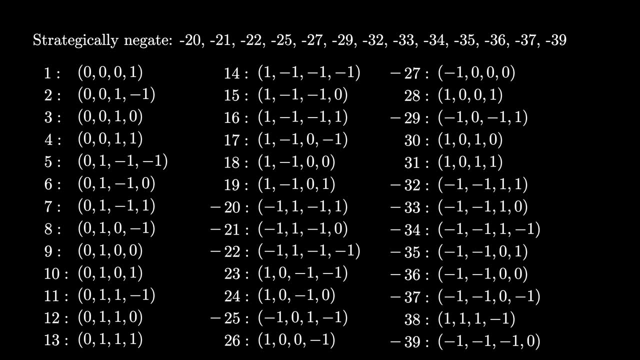 When we do these 13 values as shown here, we can strategically negate 13 values. We can then list the corresponding balanced ternary representations for these representatives and it turns out we again get a perfect balance: 13 numbers in each position have each digit of 1, a digit of 0, and a digit of negative. 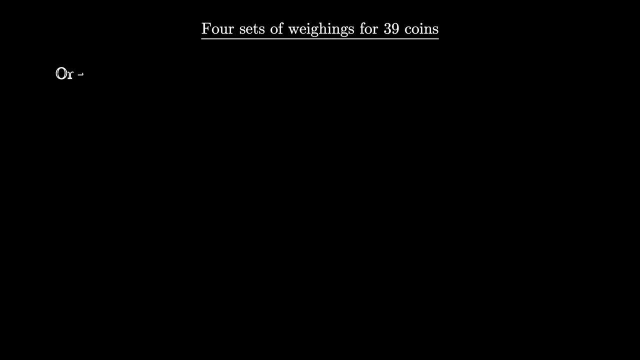 1. We can then use each of the 4 positions to create our 4 sets of weighing for the 39 coins. In the ones position, we use the numbers with a digit of 1 on the left and the numbers with a digit of negative 1 on the right. 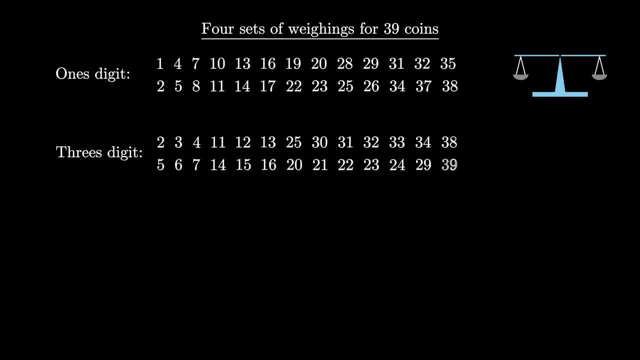 For the 3s digit, we do the same thing: The numbers with a digit of 1 on the left and those with the digit of negative 1 on the right. For the 9s digit, we have these two sets of 13,: those with the digit of 1 and those with 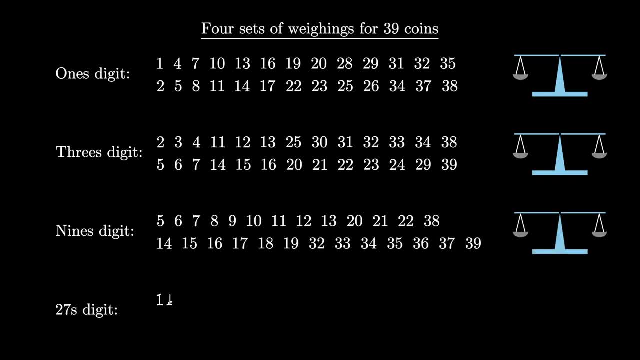 the digit of negative 1, and for the 27s digit. we have these two sets of 13 coins, As shown here. the numbers in the top set go on the left of the scale and the numbers on the bottom set go on the right of the scale. 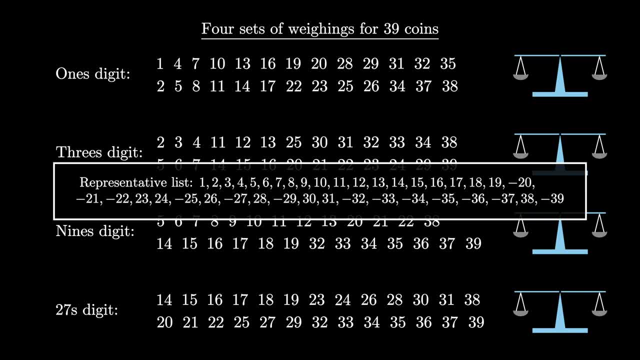 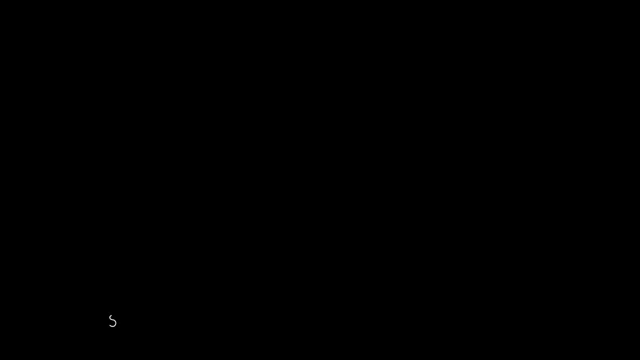 We should also remember that our representative list includes 13 negative numbers and we need to remember this list to determine if a coin is heavier or lighter than the rest. Let's see how this would work in practice. Suppose we use the four sets of weighings we just determined on 39 coins.